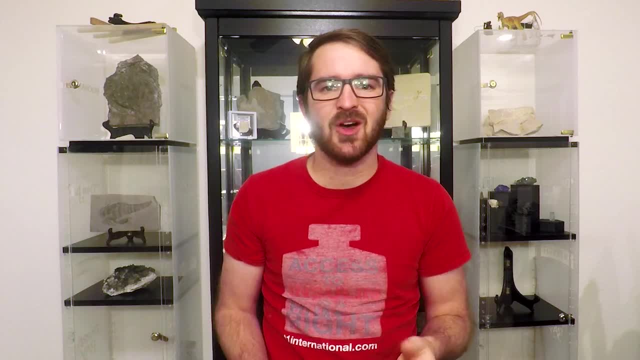 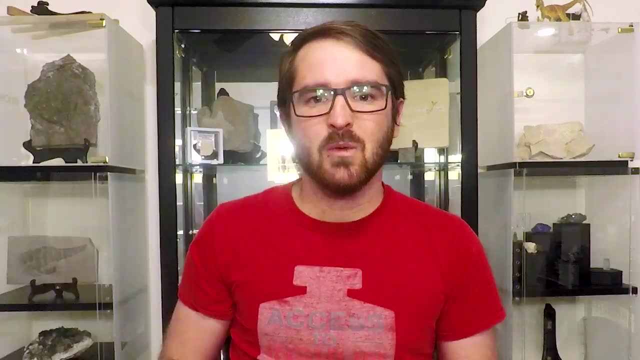 Both of these are known mostly just from teeth, and while those teeth can help us understand that, yes, there was a Spinosaur in that environment, it doesn't necessarily tell us anything detailed about the animal. What the authors suggest, because of this incompleteness of these two different genera, 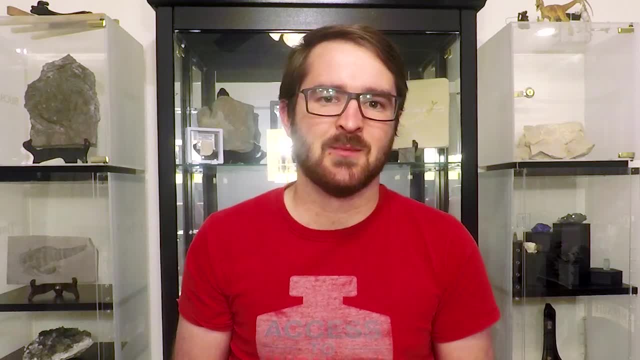 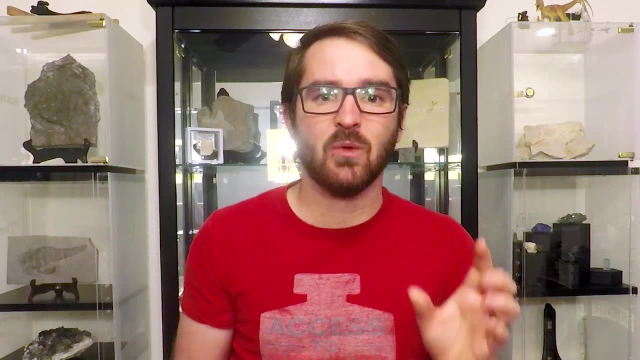 is that we shouldn't be using their names, Ostafricosaurus and Siamosaurus, because we can't identify them with anything diagnostic. Even if we found a complete skeleton of one of those animals, it would be hard to nail it down as the same thing, based solely on the 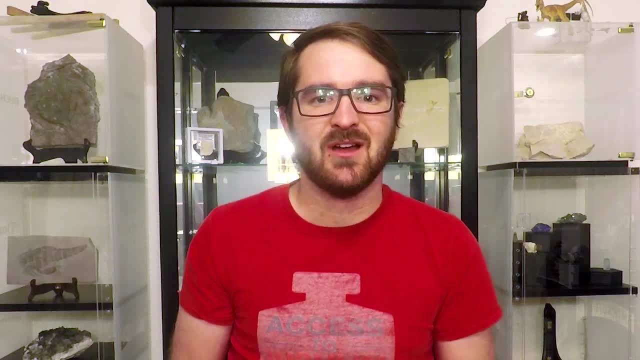 basis of the teeth. And that's because Spinosaurid teeth are very, very similar, even between very distantly related animals. And that's because Spinosaurid teeth are very, very similar, but even between very distantly related animals. And that's because Spinosaurid teeth are very, very similar, even between very distantly related animals. 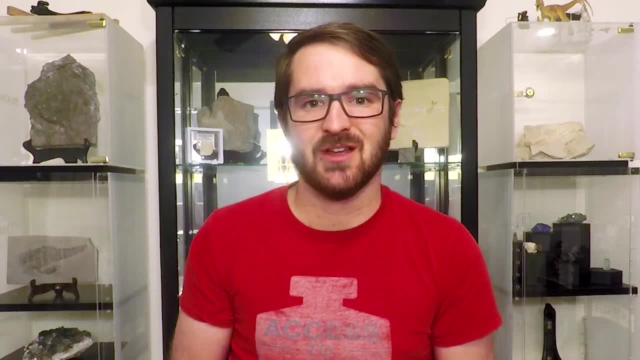 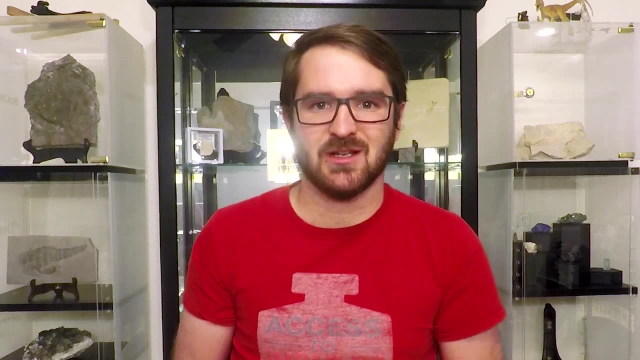 They're generally very conically shaped, useful for catching fish, but not much else And, again, not very good for diagnosing that it is a unique species or genus. Simply put, what this means is, with a lot of the Spinosaurus, we need to be very cautious. 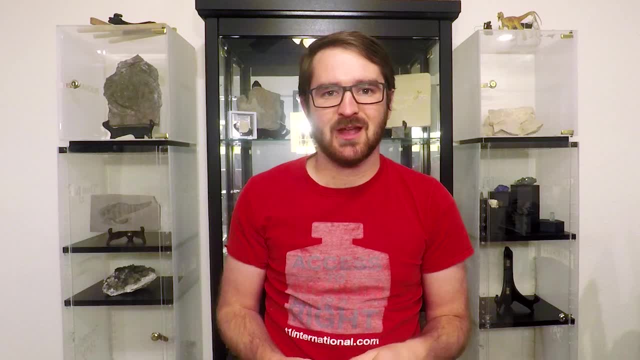 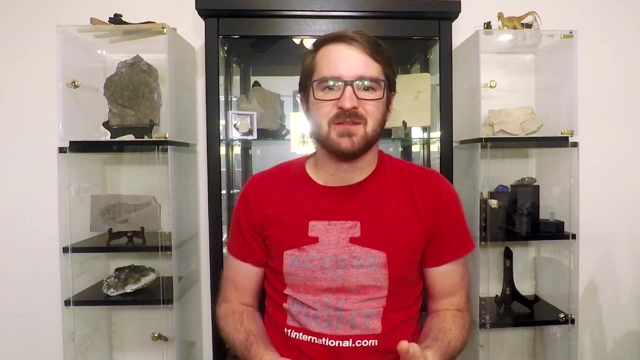 about how we group them, simply because they're very fragmentary And we need more people out there trying to find more fossils of different Spinosaurids, which so far has been slow going, mostly because they've been coming from a lot of the southern continents, which have been far less. 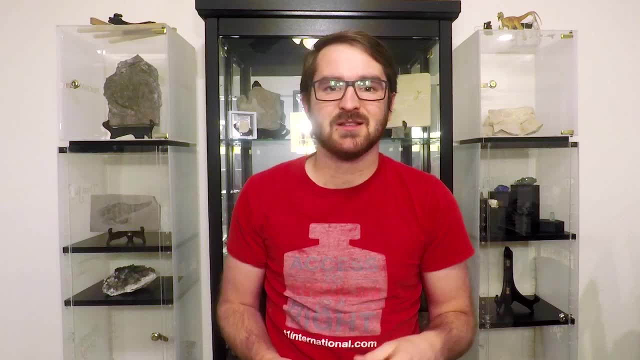 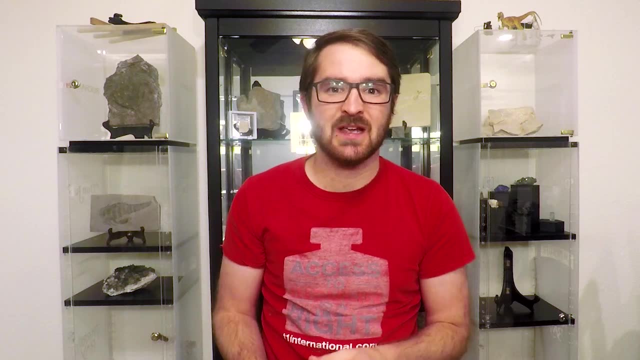 studied, in part due to how there's a northern hemisphere bias in a lot of the sciences, including geology. Another paper looked at the theropods, and the Spinosaurids with their shorter legs are kind of an outlier for this group and so don't apply as much. But the generally long 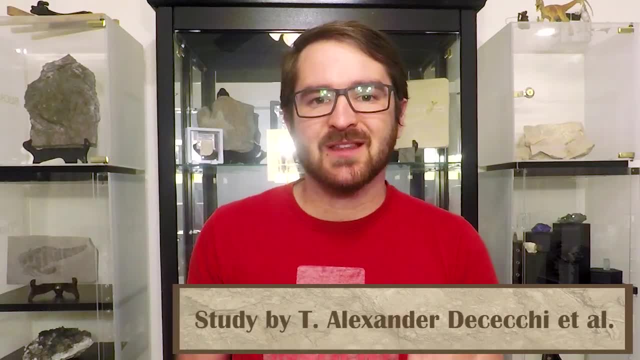 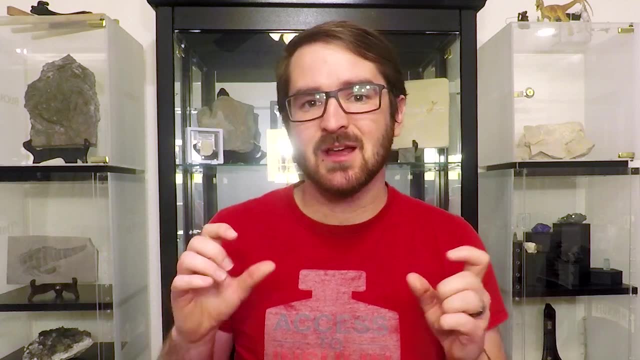 legs of the theropods are what was under study. What the study found is that the long legs of large-bodied and small-bodied theropods evolved for different reasons, Although they had the same kind of- at least visually similar- shape of being very long. What they 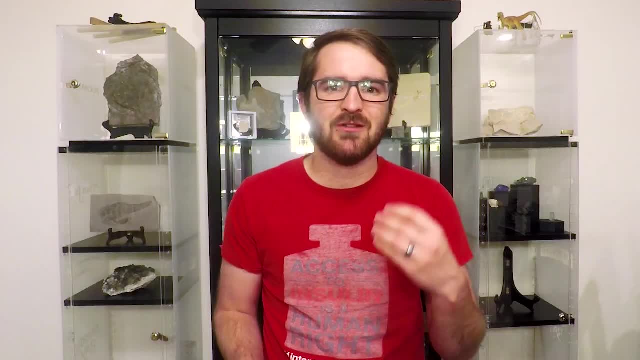 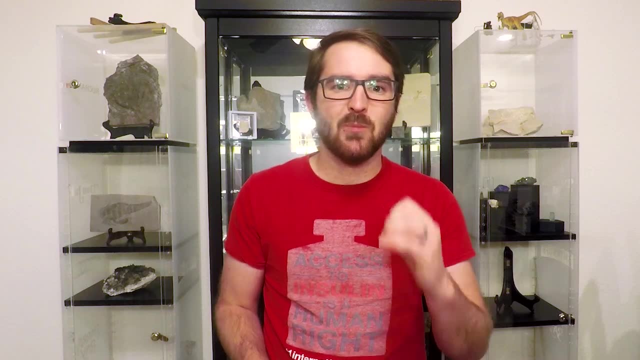 they found is that the small-bodied theropods were prioritizing trying to run fast more than trying to run efficiently, and that makes a lot of sense. They'd be catching smaller prey, which would require more captures, and more speed would help with this. However, they also could end up as 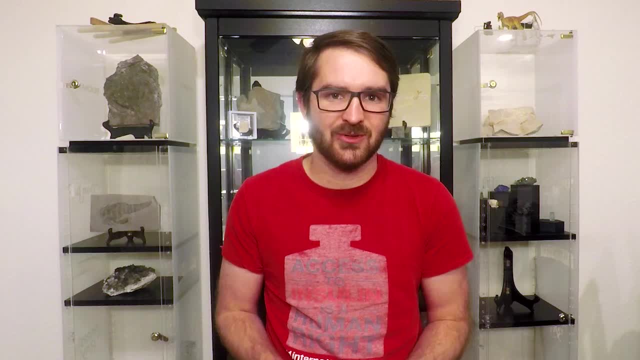 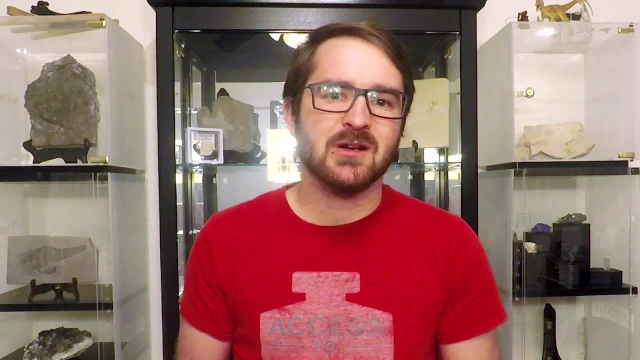 prey themselves, and being speedy to get away would be very helpful in those cases. Meanwhile, in the large theropods, which were very heavy and needed to reduce the amount of energy they used, they prioritized walking and running more efficiently, particularly in the tyrannosaurids, which saw a 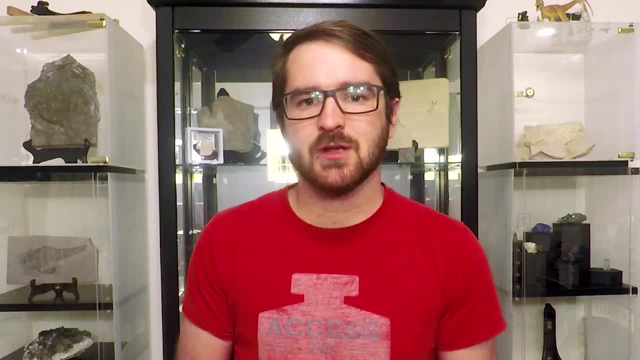 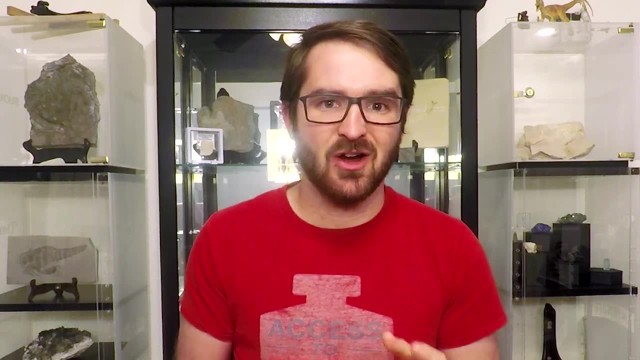 very, very efficient leg gate over more basal kinds of carnivores such as Acrocanthosaurus, which formerly was the dominant predator of North America up until the tyrannosaurids arrived on the continent. What this suggests is a very symmetric curve for the speeds of theropods. 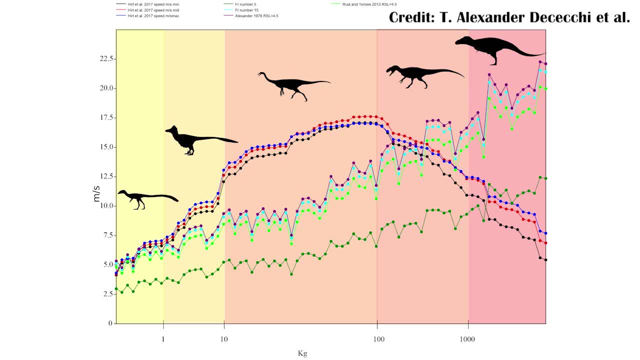 With the smaller theropods prioritizing speed. they're still very much smaller than the mesoarcher animals, meaning that even with relatively long legs, they still won't be able to take as long of stride lengths as the larger theropods. 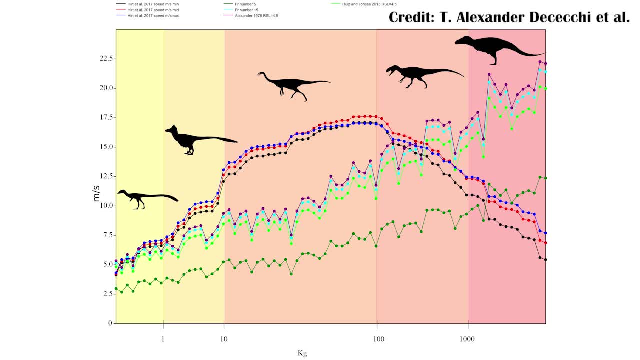 but their speed is going to prioritize them, slightly higher than they would be otherwise. Meanwhile, the medium-sized theropods are prioritizing both, but since they do have that medium body size, they can take longer stride lengths and attain a higher speed. And then the 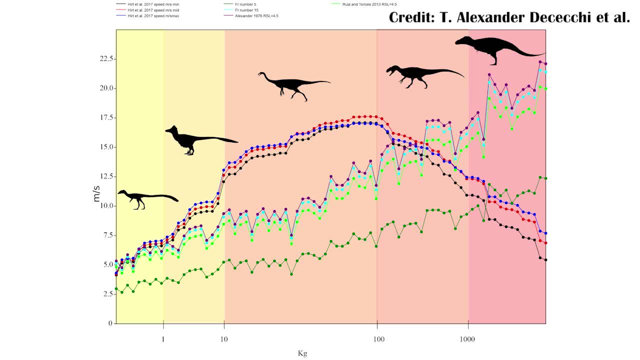 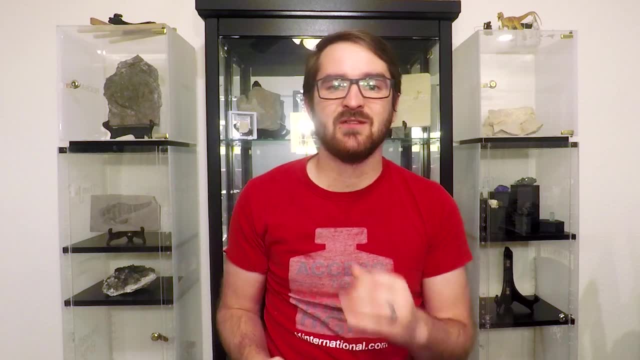 speeds drop off again with the larger theropods, making this very symmetrical graph of the speeds versus body size in the theropods Still on the theropods Allosaurus represents one of the best known tactics in the world of theropods, which is to say that they are the most powerful and 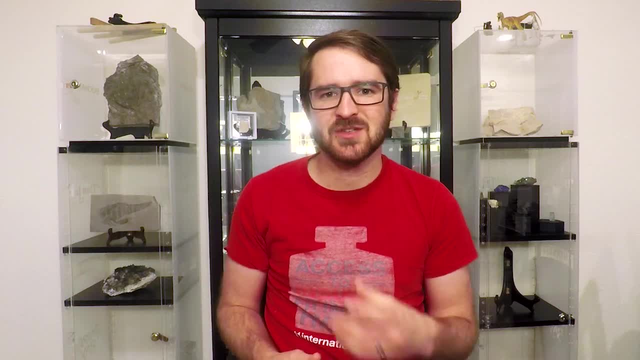 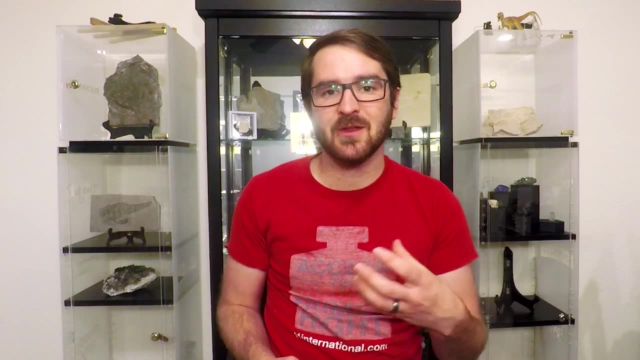 aggressive of the theropods in North America, And this is because of many fossil sites that, essentially, would have acted as predator death traps. An animal would become stuck in it and theropods would come around from the area in order to try and feed on that easy prey. 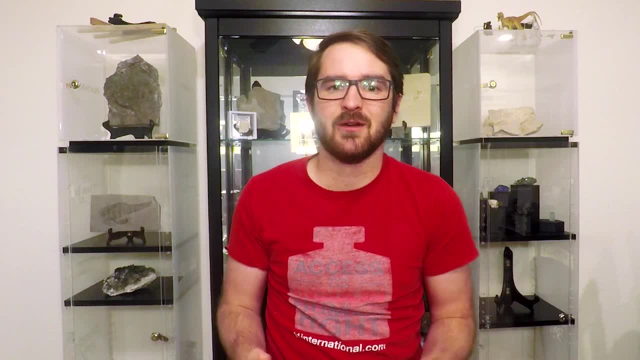 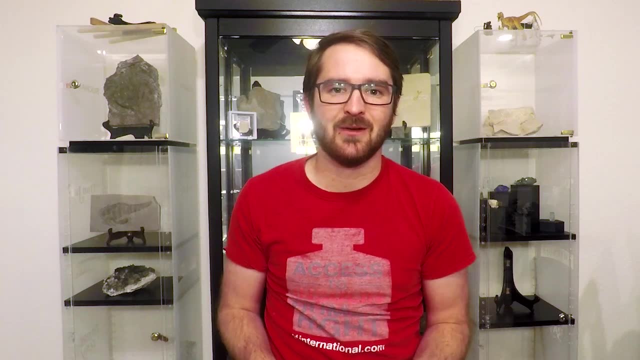 They too would become stuck in whatever kind of muck or bog there was and then also become fossilized. This is very similar to the idea behind the La Brea Tar Pits in LA County. The Migat Moore Quarry in Western Colorado is one such site where. 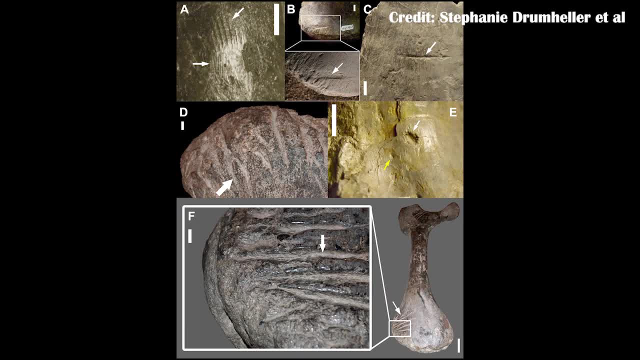 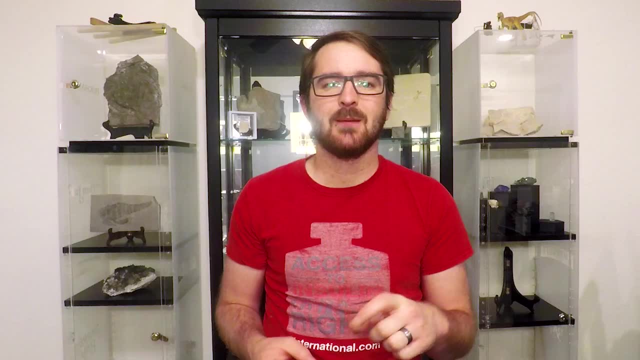 a plentitude of Allosaurus found. What fossil studies have shown from this site is bite marks on both the theropods that were stuck there, but also some of the Allosaurus. By studying where the bite marks occurred on the animal, it helps us to understand exactly what kind of behaviors. 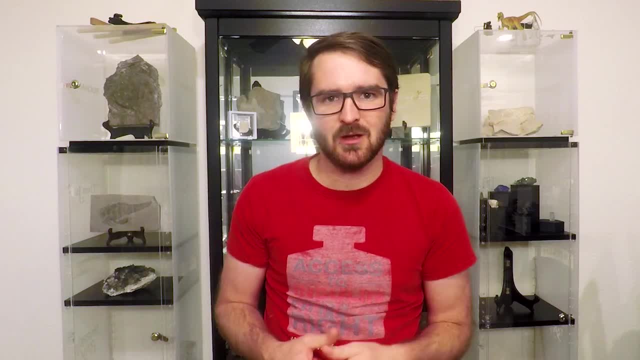 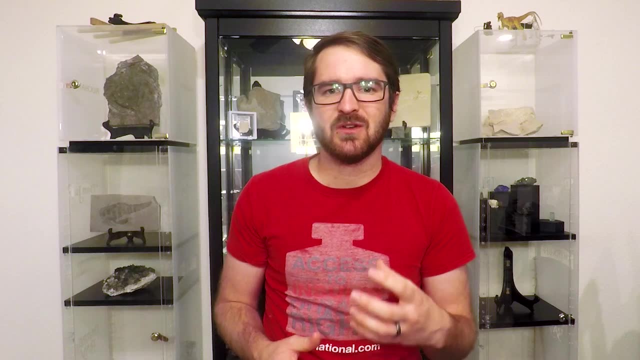 may have gone into this kind of biting and interspecies combat. What it suggests, though, is that about half the bites were from areas that were highly nutritious, meaning it would have been more meat and muscle, making it more healthy for the animal to survive, And that's what we're. 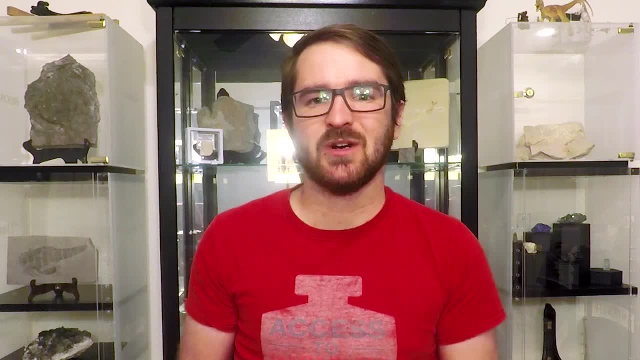 looking for. This also means, though, that about half the bites were in less prominent places for this kind of feeding, meaning it would have been things like the tail which had less meat on it. What this suggests is that may have been more interspecies combat, but the bites on the highly. 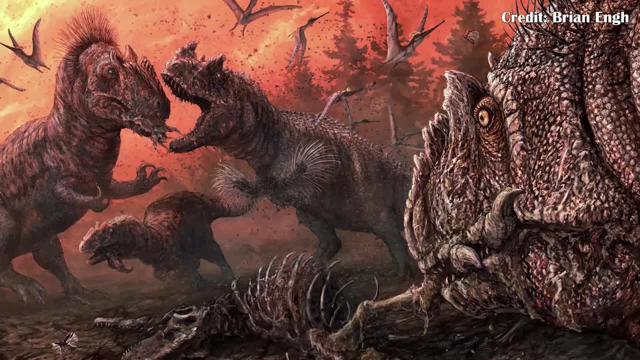 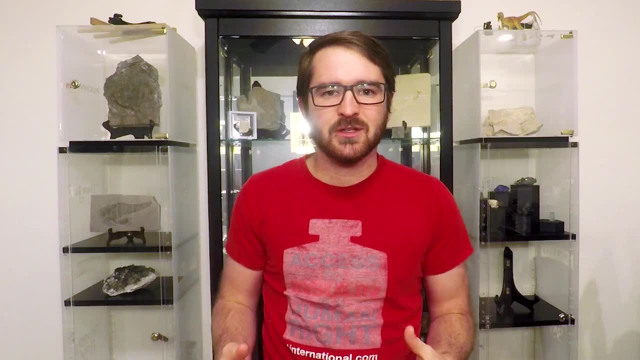 nutritious parts do suggest that Allosaurus was, at least sometimes, a cannibal, which makes sense. Allosaurus was a meat eater and, incidentally, is also made of meat. It is also important to note, though, that the study did also look at the bite marks on some of the sauropods. stuck there and found that a higher percentage of the bites occurred on sauropod bones and also were in the more nutritious parts of the sauropod, meaning that that was more primarily a food source rather than just some interspecies of competition that occasionally turned to cannibalism. So Allosaurus wasn't necessarily using other Allosaurus as a primary food source, but it certainly wouldn't miss the opportunity if it needed it. As for other North American dinosaurs, there have been a lot of new finds coming from the Prince of northern Alaska, including some dinosaurs that would have lived very close or above the. 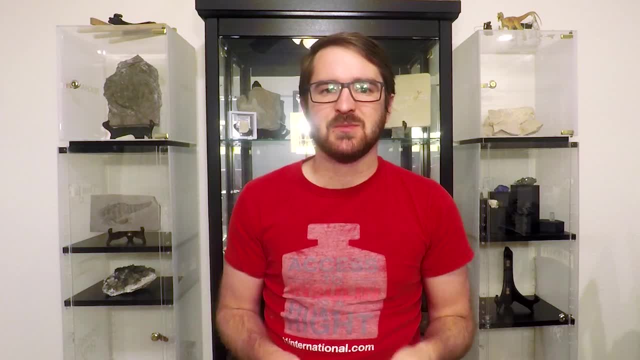 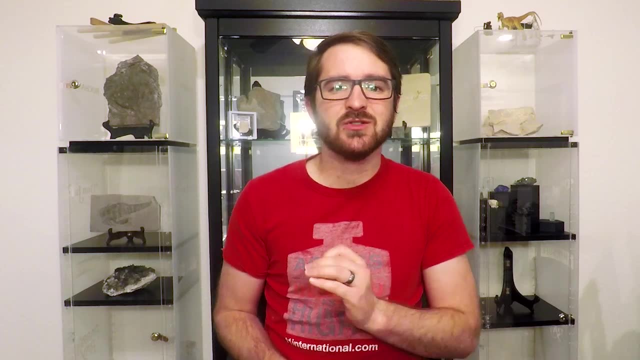 arctic circle. Many of these animals have been thought to be their own unique species, but a new study suggests that at least one of them wasn't. A juvenile hadrosaur has been shown to have no discernible differences from Edmontosaurus, meaning that, for all practical, 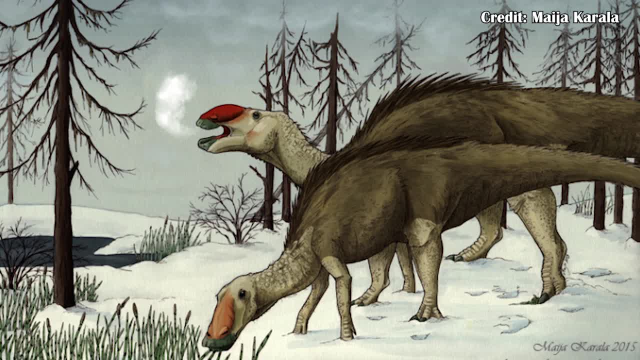 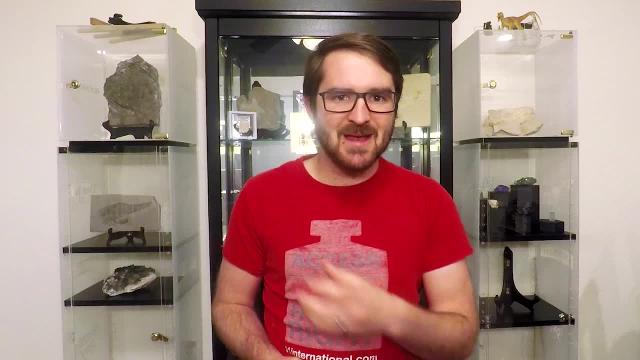 purposes, it is an Edmontosaurus until it can be proven otherwise with a more adult specimen. Edmontosaurus is ending up being one of the most widespread genera that we know of, coming from many different sites across North America during the end Cretaceous. 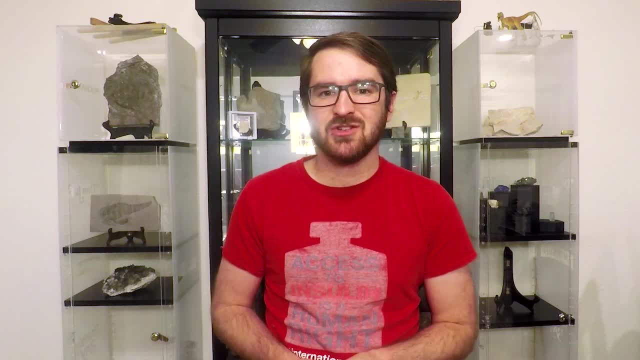 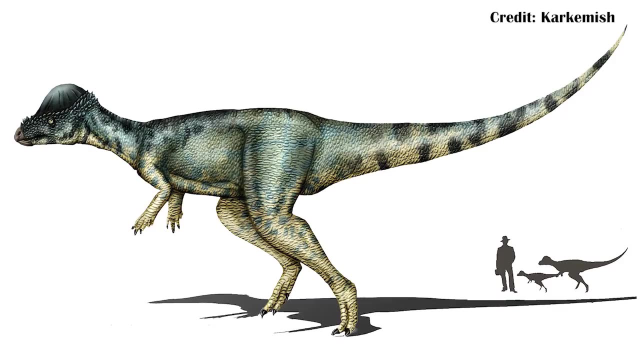 And with so many very fragmentary fossils coming from the Prince Creek Formation, it's possible that many of the species named from there, such as Nonoxorus or Alaska Cephalae, may just be other species that are known from elsewhere in North America. However, 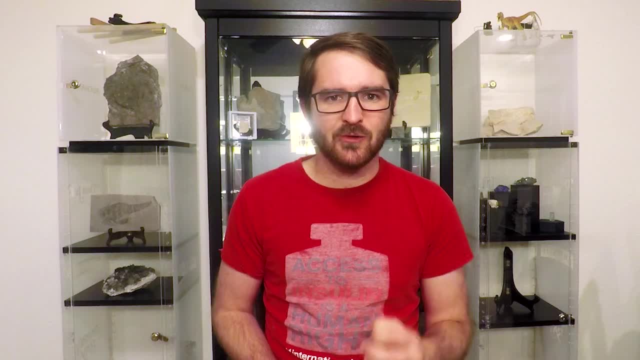 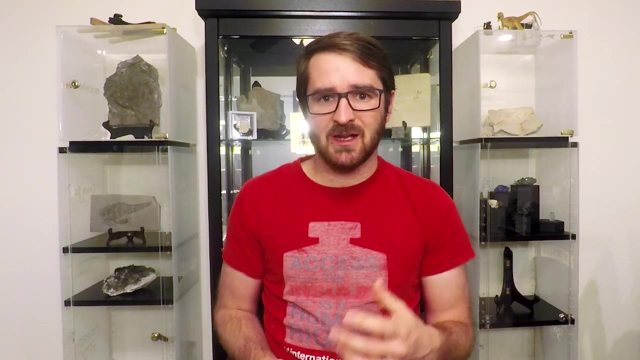 it is going to take more fossils coming from this formation in order for us to understand just how diverse and widespread the Edmontosaurus is, The different very northern dinosaurs were, and just how unique or non-unique this environment may have been. Edmontosaurus lived until the very end of the Cretaceous meaning it would 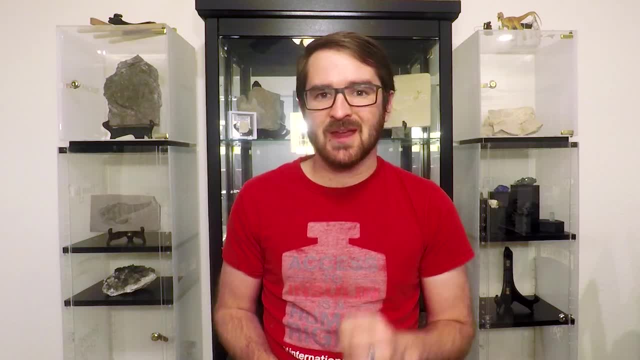 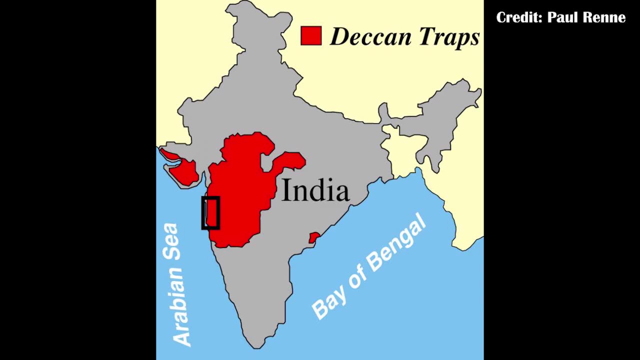 have seen meteors strike the earth, And a new study is showing that without that meteor, the extinction probably wouldn't have happened. The Deccan Traps in India were a set of massive volcanoes, and it's been hypothesized that while these were erupting, at the very end of the 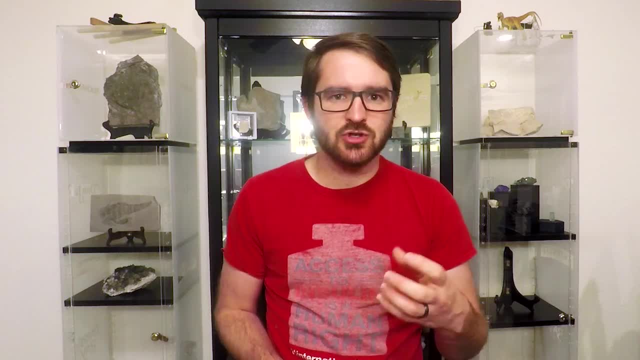 Cretaceous. they may have caused a change in the climate which could have caused the extinction on a much larger scale. So if you're interested in learning more about the extinction of Edmontosaurus, you can click on the link in the description below. 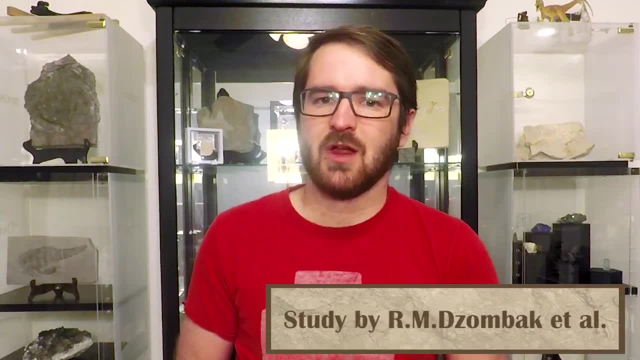 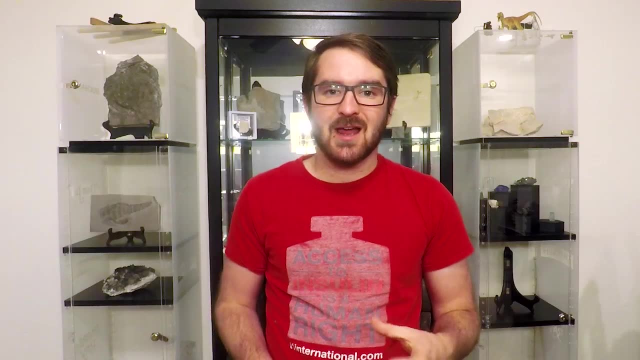 A new study sought to try and see what happened to the local climate in India while these eruptions were occurring, and what they found is that there was generally not a major change. India during this time was dominated by rivers and forests, and what the study found is that 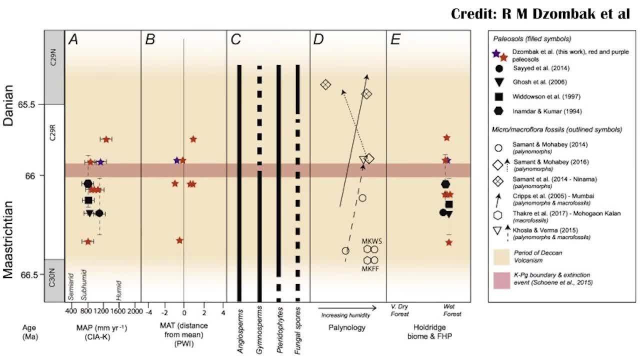 there wasn't much change in this during the time of the eruptions, meaning that even though these were very, very massive eruptions, they didn't have nearly the same kind of significant impact on the climate as the Siberian Traps did during the Permian-Triassic extinction. 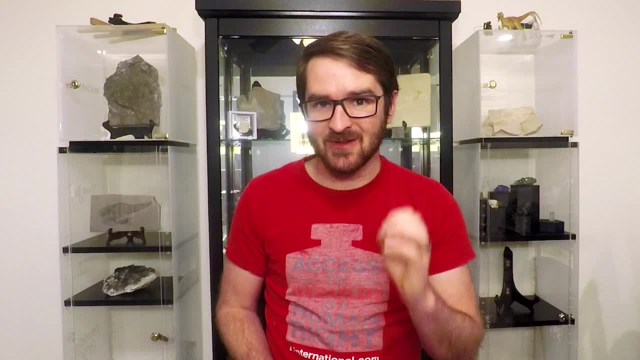 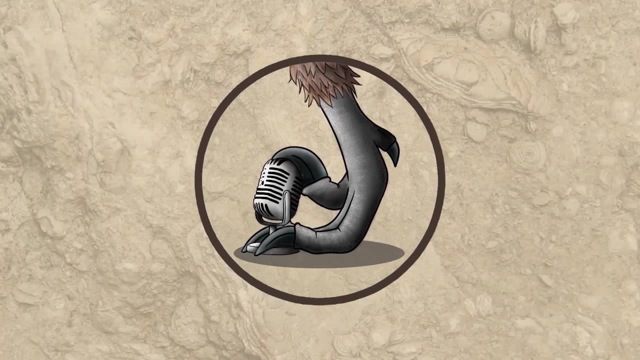 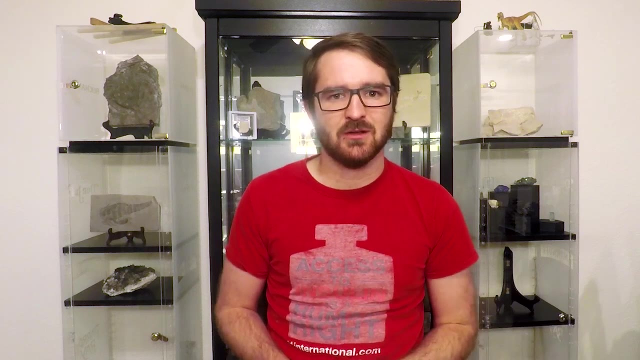 What this means is that it was very much more likely to be the meteor as the main cause of extinction rather than some environmental change during the time. As for that impact, a new study has suggested that it happened at the wrong angle and became even more devastating because of that angle. What the study found is that the 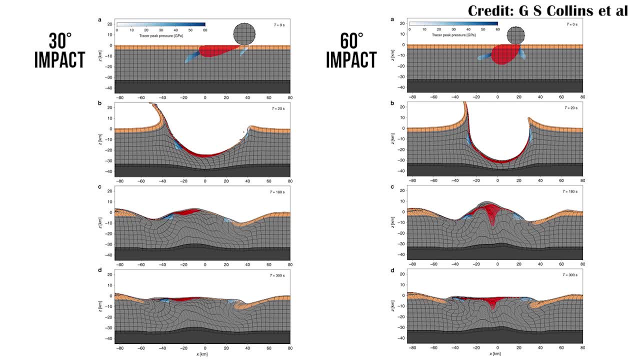 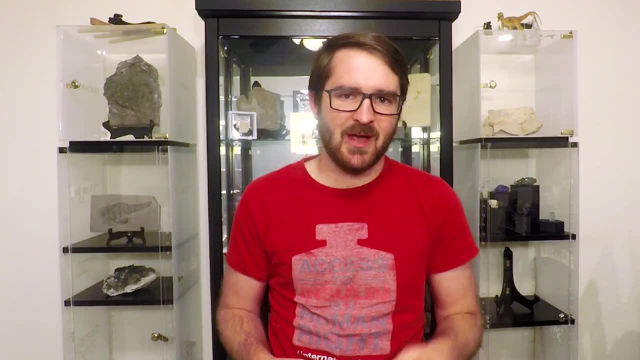 impactor came in at an angle of higher than 60 degrees, which most meteors don't do. This very high angle only occurs in about one-fourth of all impacts that have happened on the planet, And it would have been able to then launch a lot more of the vaporized gases of the very sulfur-rich rock into the atmosphere. While the impact itself would have created a massive wave of heat, these gases high in the atmosphere would have blocked out a lot of sunlight, creating a kind of nuclear winter, except caused by a meteor rather than nuclear explosions. 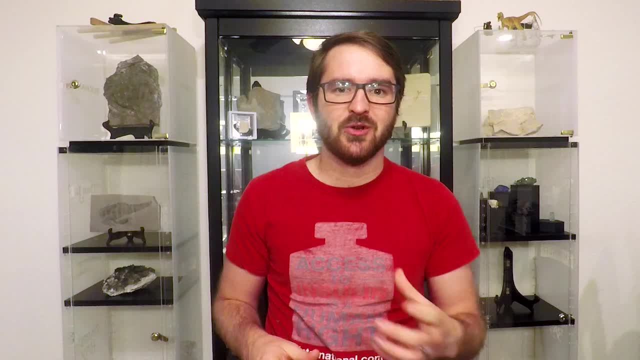 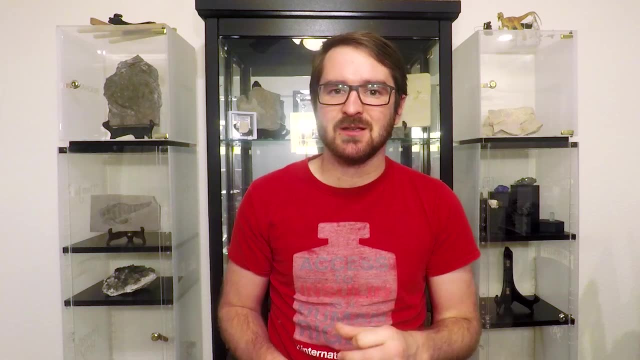 There have been other studies that do suggest that this sulfur-rich rock was also a major part of why the extinction happened, meaning that there were many factors that went into this extinction being as severe as it was and leading to the eventual evolution of humankind. 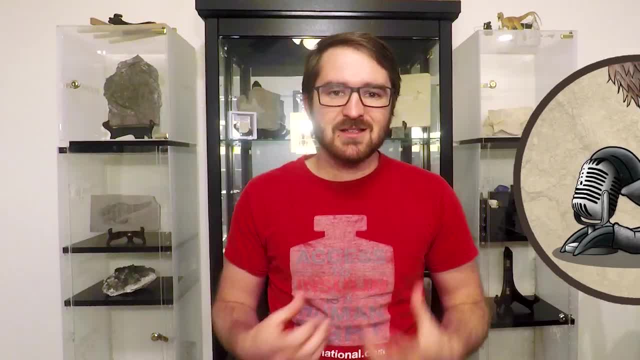 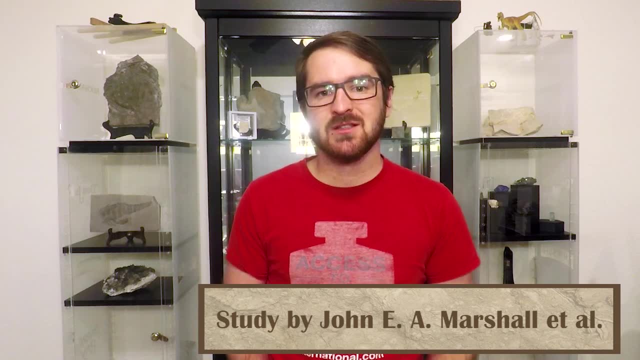 I mean, we were very lucky to even show up. A less talked about extinction is the one that occurred at the end of the Devonian period. A new study has suggested that a major cause of this extinction was UVB radiation coming from the sun. What happens with UVB radiation? because it's 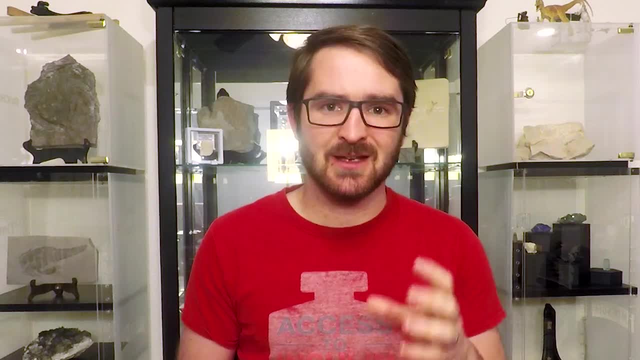 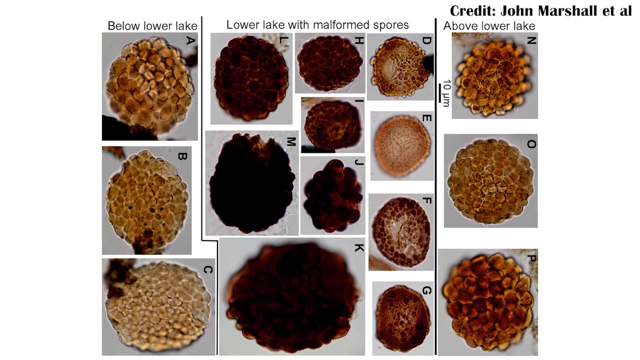 so high energy is that it can mutate certain seeds and different pollens from plants. Controls with modern-day plants have shown a lot of these shapes and the fossilized pollen and seeds show these same identical shapes, meaning that they were mutated in the same way, likely also by UVB radiation, Normally the ozone layer. 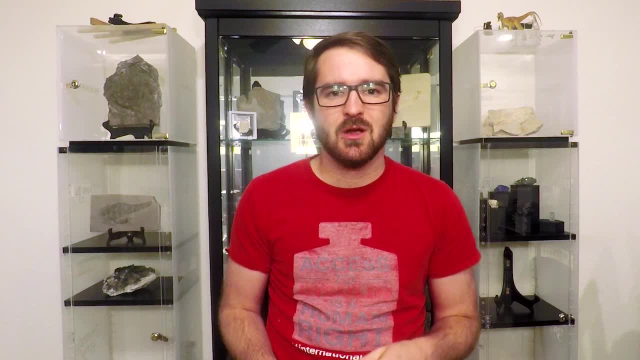 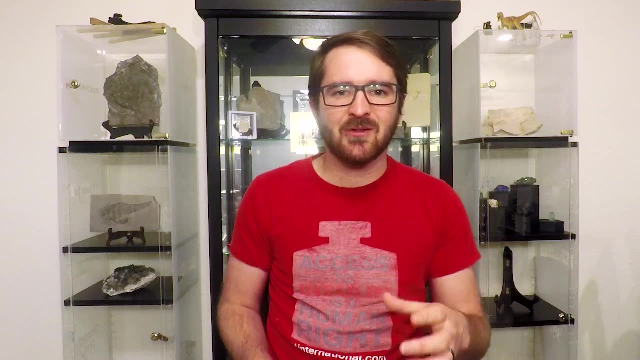 protects from a major part of the UVB radiation, meaning that there's not a significant risk of this kind of thing happening as long as we keep the ozone layer intact. However, the study also points towards global warming that occurred at the end of the Devonian and suggests that ozone 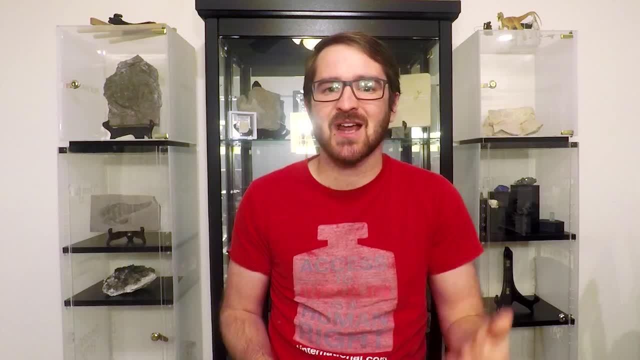 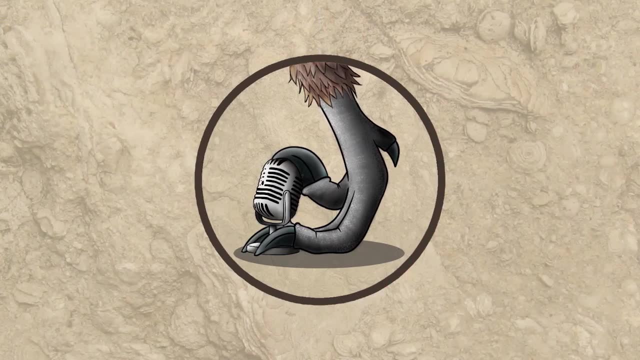 layer decay may occur as just a natural side effect of global warming, meaning it is something that we should be concerned about and keeping an eye on towards the future. One of the groups that did survive this extinction at the end of the Devonian were the Eurypterids. The Eurypterids- 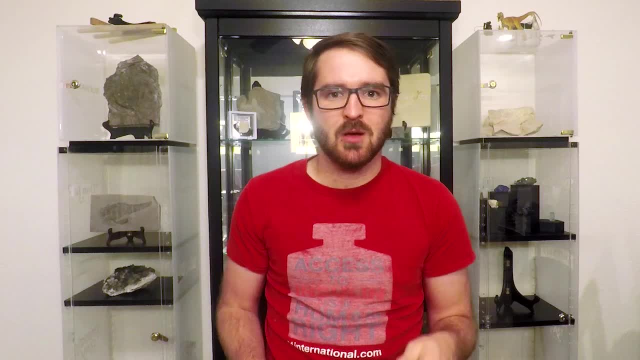 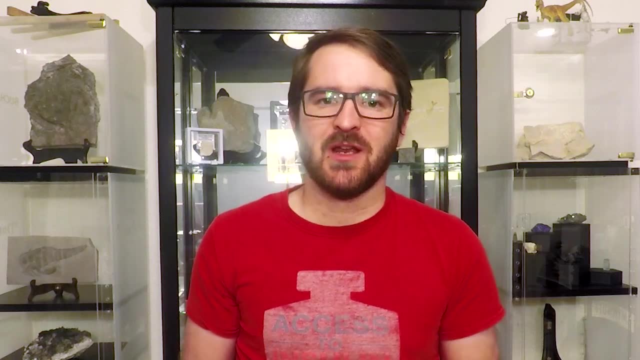 are also called sea scorpions, and they aren't true scorpions but are related in a larger family, though they're not quite arachnids. Some of these Eurypterids did what is known as sweet feeding, meaning they had long arms with different fronds at the 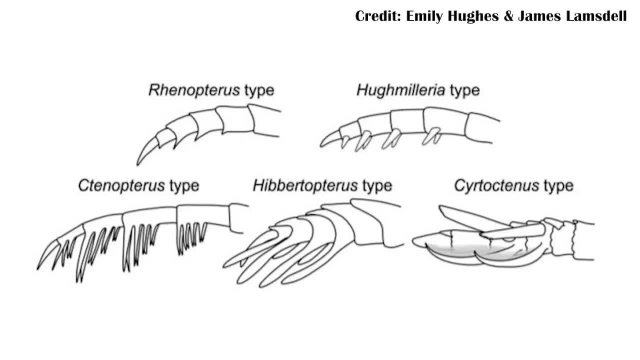 top of their heads, and they had long arms with different fronds at the top of their heads and tips of them that they would use to sweep food into the mouth, While many of the arms on these different animals did have different types of tips at the end of them which would have selected for. 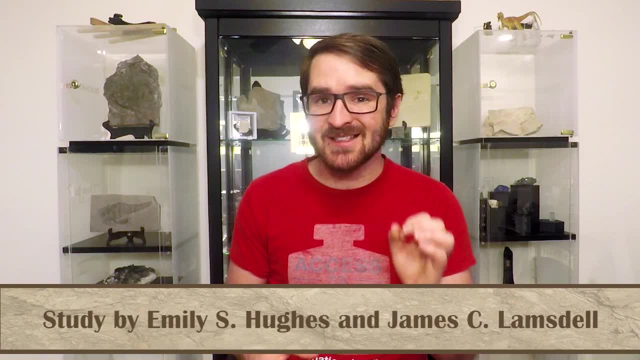 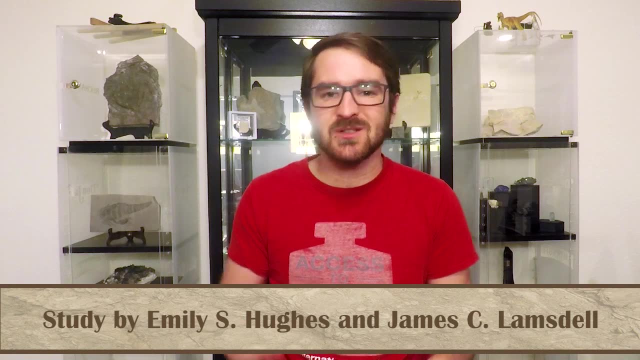 different types of food. what the researchers found was that this different type of food preference had no impact on whether or not the animals went extinct at the end of the Devonian or succeeded beyond it. Instead, it was much more likely location, at least based on what this study. 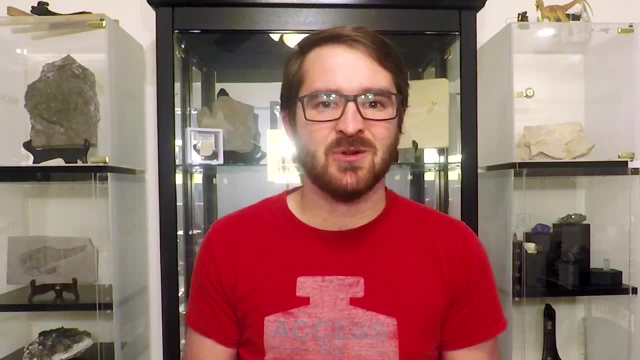 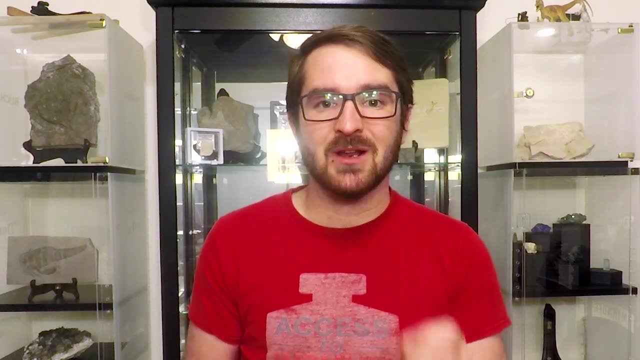 found. The researchers were specifically trying to test if the different food choices did have an impact on the animals, and while that hypothesis was proven wrong, it does help to show how testing these hypotheses, even when wrong, can help us to understand much more broadly about the animals and help us to develop new ideas about why they may or may not have gone extinct. Another: 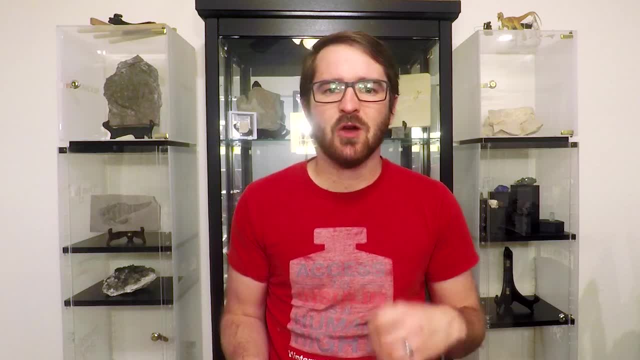 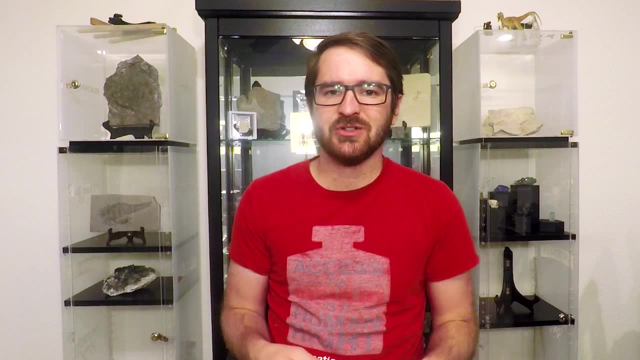 group that didn't fare well during the end Devonian extinction was a group called the Placoderms, which included some of the largest predators in the oceans at that time, such as Dunkleosteus. One of the close relatives of the Placoderms was the Placoderms, which included some of the largest predators in the oceans at that time, such as Dunkleosteus. One of the close relatives of Dunkleosteus was Titanichthys, which has generally been considered very similar with a very similar body size. However, a new study on its jaws suggests at least, as some people had started to. 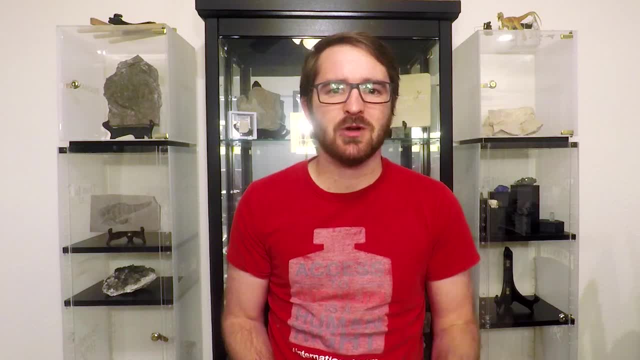 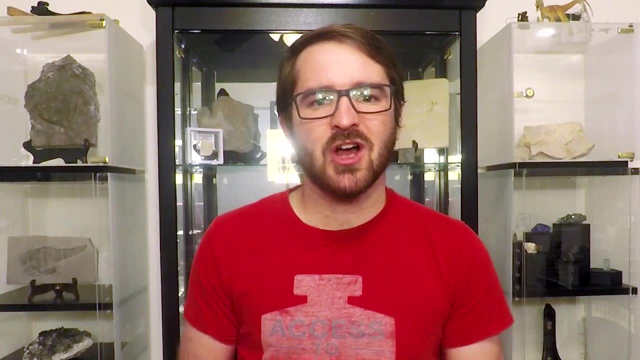 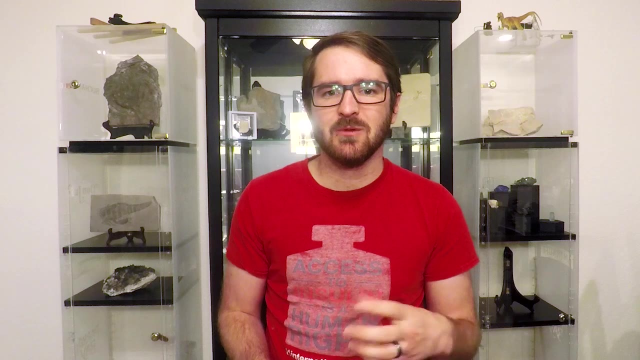 hypothesize that it may not have been much of a predator, instead being a filter feeder. The jaws of Titanichthys actually line up fairly similarly with the jaws of the modern basking shark, which is a large-bodied filter feeder. If Titanichthys was a filter feeder, it would show the 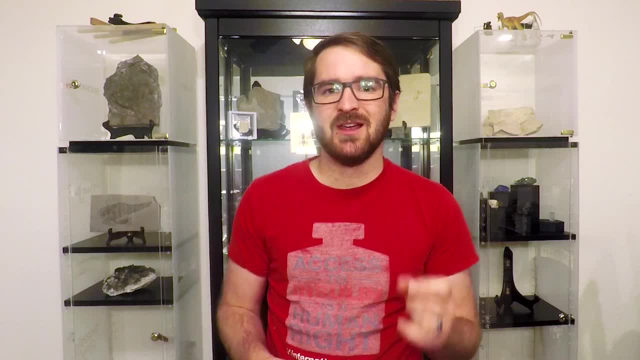 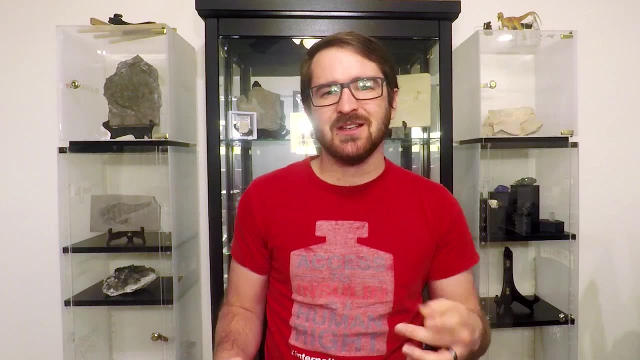 evidence of the first very large-bodied filter feeder in the fossil record, meaning that this niche was occupied very early in Earth's history. Extinction events can also lead to very rapid radiation and very unique designs occurring in the fossil record. What one of these radiations led to? 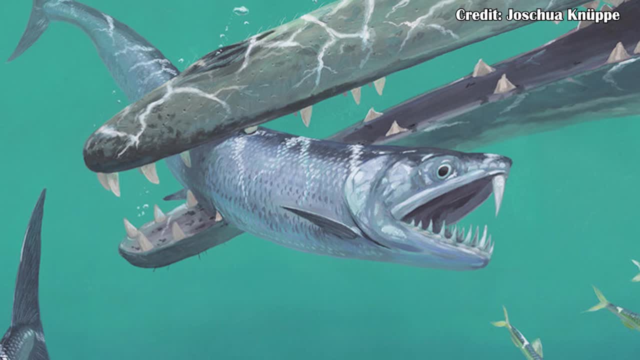 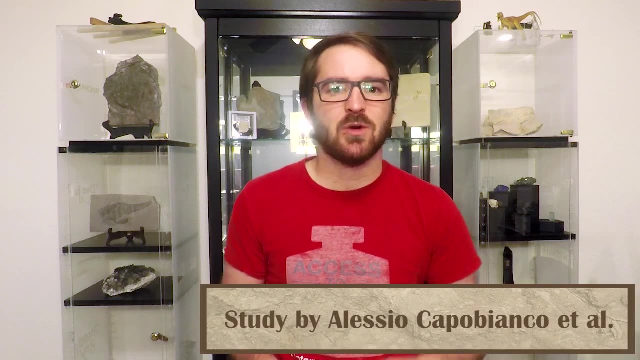 was a saber-toothed anchovy that was almost three times longer than any of its close relatives. Modern anchovies are very small filter feeders, but this one would have been much more of a predator, having more teeth than just the size of a fish. Titanichthys was a very large-bodied filter feeder. 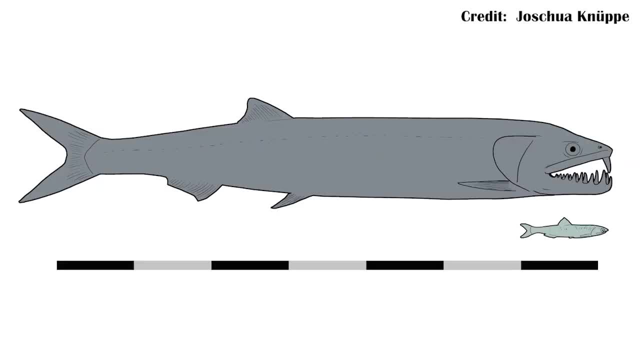 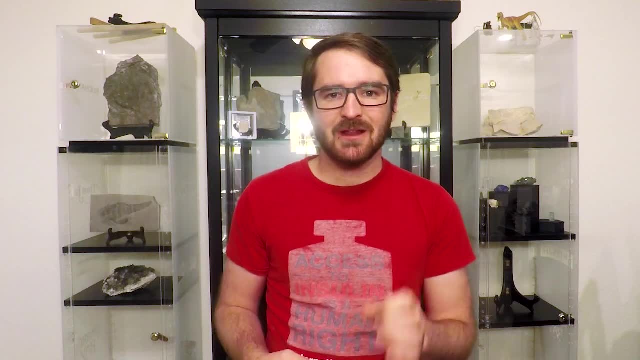 with a single saber tooth that would have been at the front of the mouth and also having a much larger size again, being about three times larger, meaning they would have been close to a meter. Unfortunately, these animals did die out, likely due to competition with many of the modern predatory. 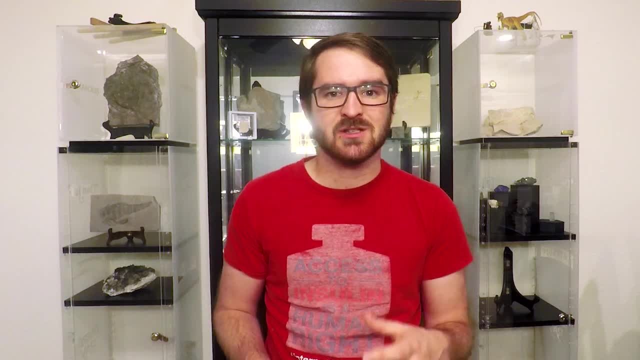 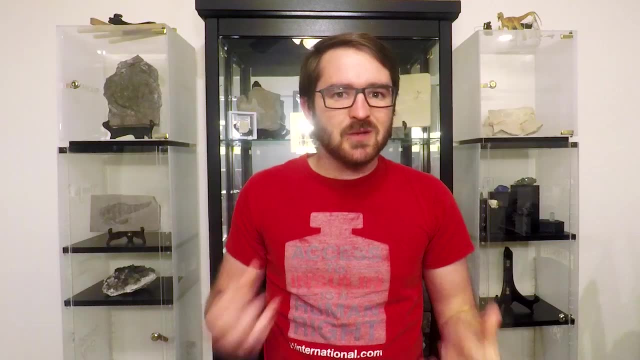 fish clades that were also diversifying at the same time, such as some of the first tuna and billfish, which obviously became much more successful than the predatory anchovies. On the subject of teeth, a study of the teeth of Deinonychus suggests that it probably was not a pack hunter Oftentimes. 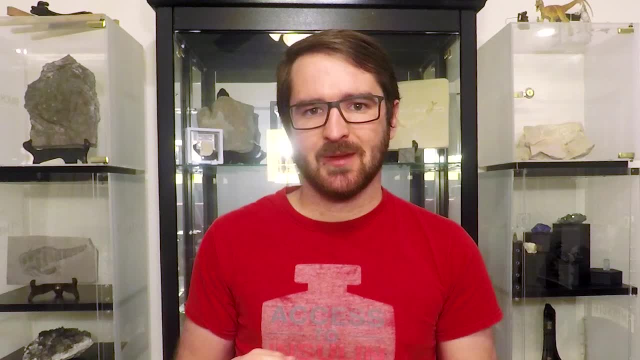 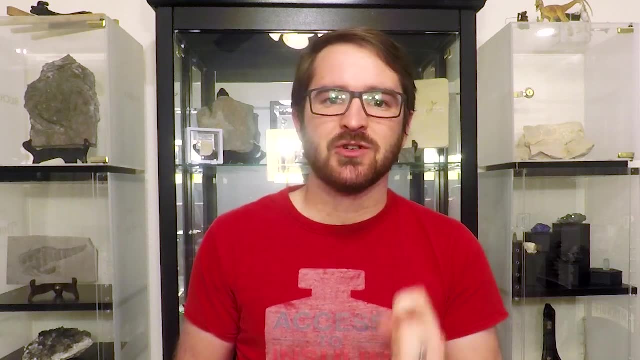 with teeth, the enamel can be so resilient over time that it's the exact same enamel that the animal originally had. By looking at the teeth of Deinonychus, some of the isotopes preserved in there have been found, specifically oxygen and carbon isotopes. The isotopes in the enamel will have 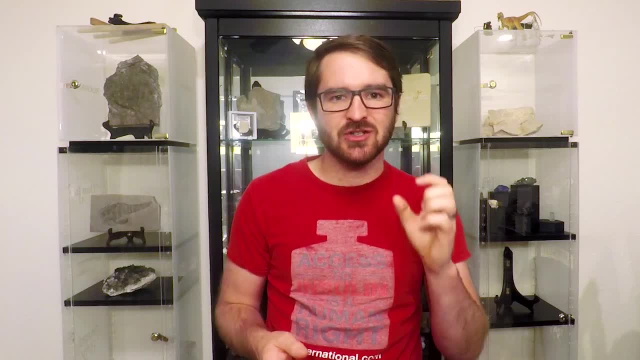 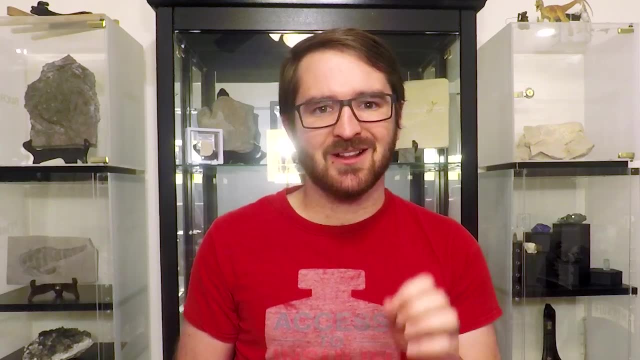 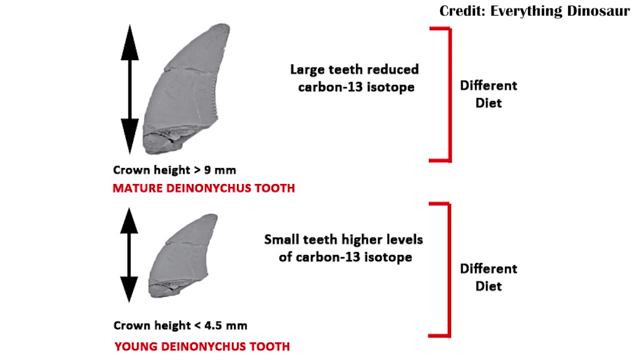 different biases depending on what food source the animal is trying to choose and be deliberately selecting towards. The study looked at teeth of Deinonychus coming from the antlers and cloverly formations of Montana. What they found is that the teeth have different selection biases towards different isotopes. 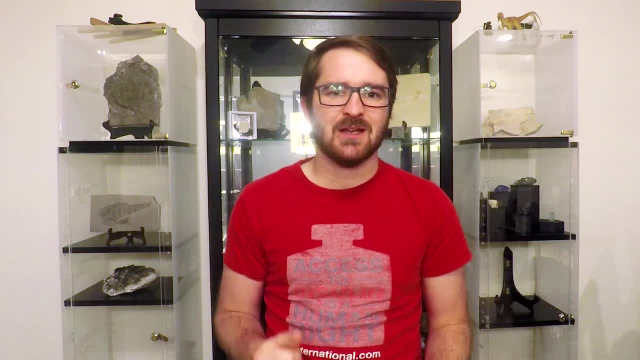 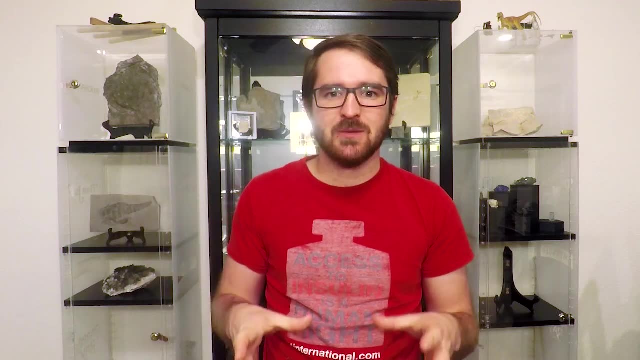 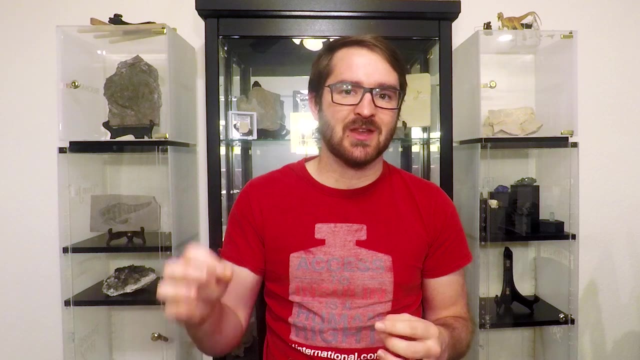 depending on the size of the animal. This is not what you would expect if it was a pack hunting animal. In a pack hunting animal, the entire group of that pack is going to be selecting towards the same foods, meaning that their teeth will develop the same biases towards certain isotopes that are 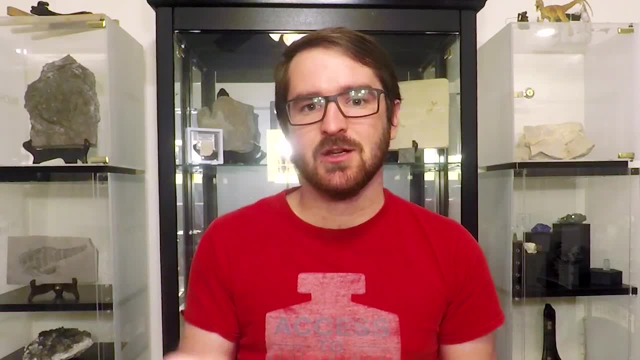 found in that food source. Because the teeth of Deinonychus show different isotope biases over time, they are not going to be selected towards the same food source. They are going to be selected towards another food source as well. but those style of influences are not going to be desserts as well. 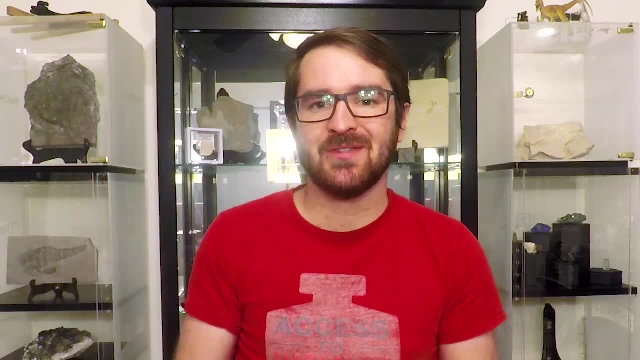 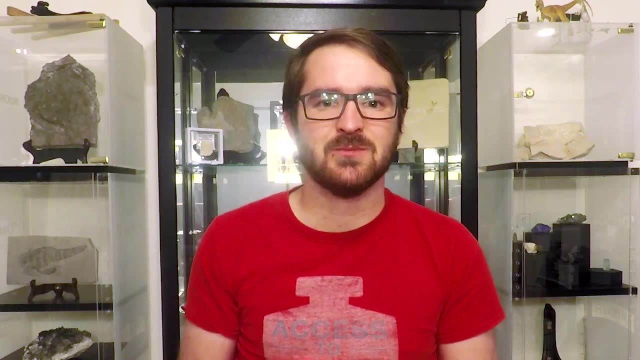 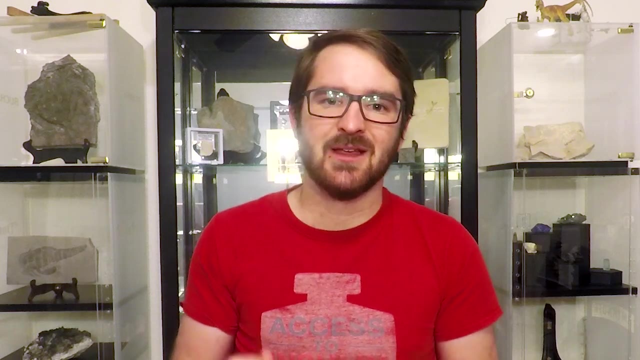 What Tinnontosaurus also found is the teething bias. During the same year, as the animal was very young- to find habitat for the Tinnontosaurus, I found some of the teething biases that were found at the same plant company, A Tinnontosaurus from then 分. 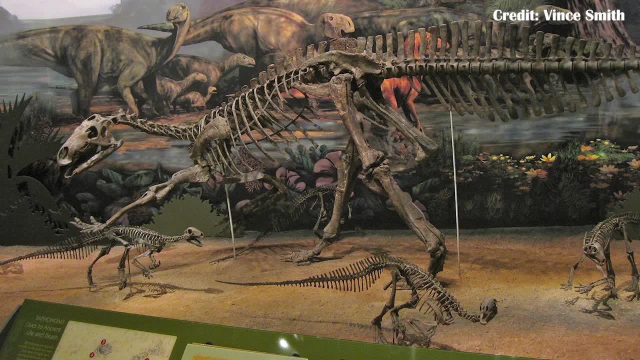 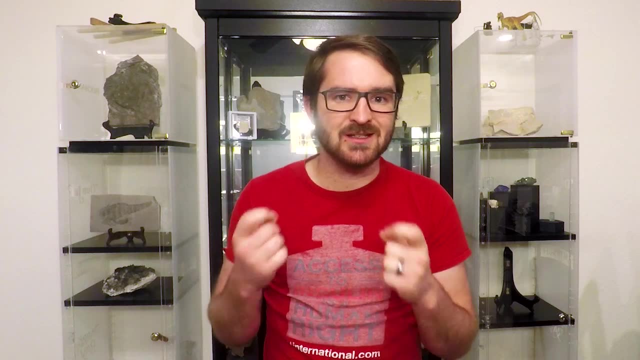 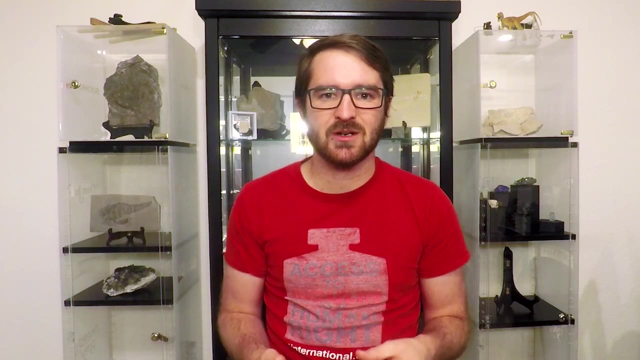 Tinnontosaurus from then uted, but really there were no biases or traces- or that's not attempting- from these. individuals show no significant bias towards different types of isotopes in the teeth, meaning they would have very likely been selecting from the same food sources. something to be more. 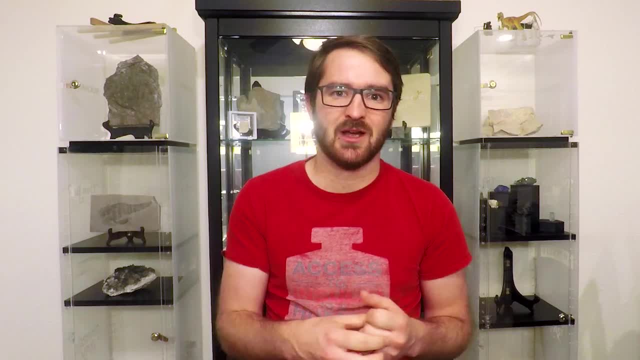 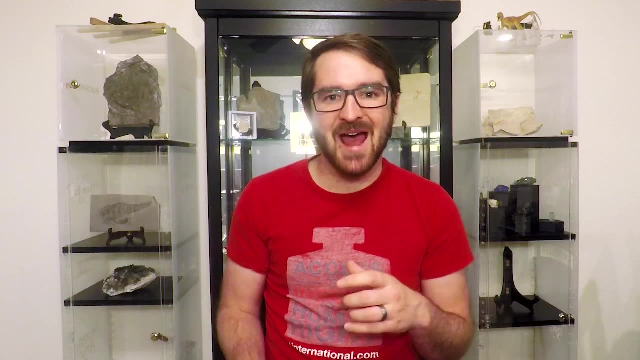 expected in an animal that is directly raising a juvenile. What this means again is Deinonychus was very much more likely like a crocodile, meaning they would have had still some defensive behaviors towards their young, but not to any significant degree, as it would have been much. 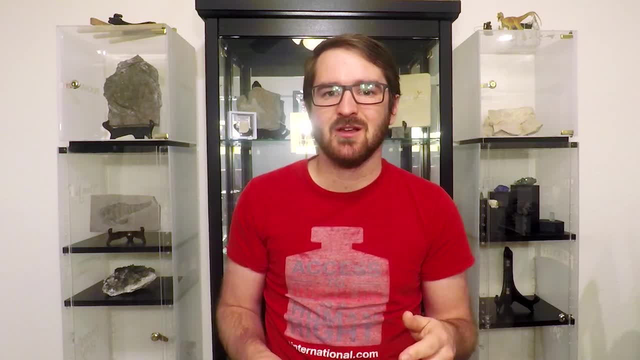 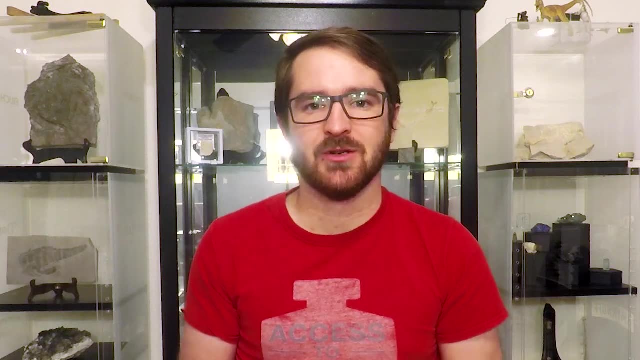 more likely that they were essentially protecting them in the same environment rather than directly feeding them with the same food sources. It's also important to remember, though, that this is just one case, in the raptors, of not being pack hunting. The Utah raptor block, coming from Utah, shows many different individuals of different ages coming from a single nine ton sandstone block. That block still needs to be studied in greater detail, though, so there is still a chance that some of the raptors and dromaeosaurs did do some level of pack hunting. 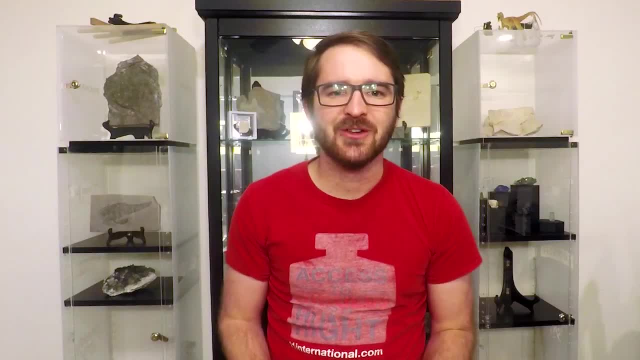 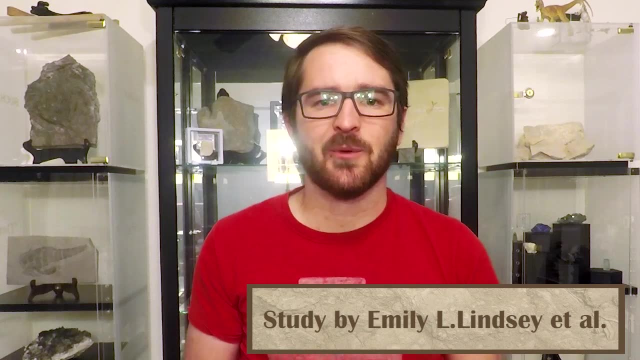 It's just not that likely. in Deinonychus, though, New fossils from a more recent time, though, do show an animal that may have lived in groups, and that's giant ground sloths. A new find coming from Ecuador shows many different ages of ground sloths, all living together in the same environment. These 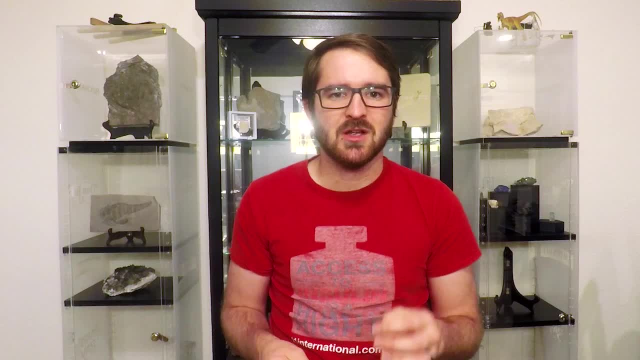 were asphaltic sediments, meaning that they would have been somewhat similar to the little brea tar pits. However, the fact that there are also coprolites coming from these sediments suggests that it wasn't quite as sticky and they may have actually been wallowing in this kind of. 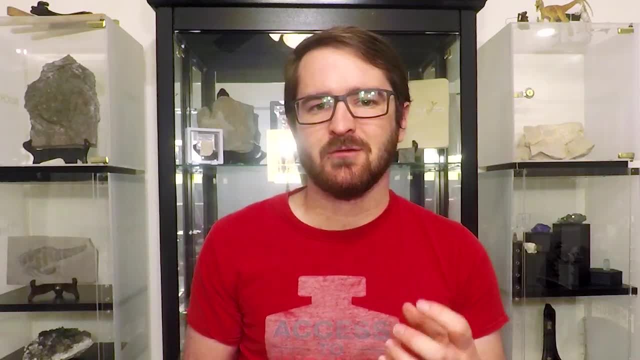 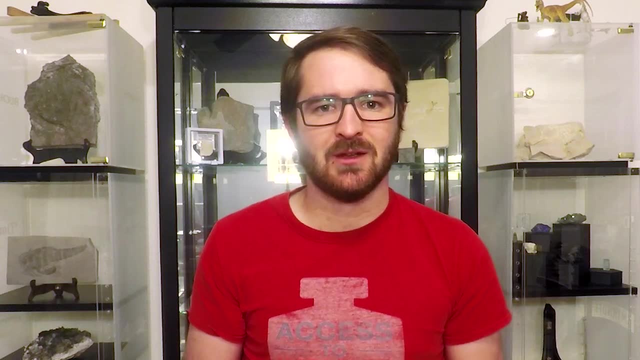 damp, oily environment. As much as it may seem strange to think of ground sloths as something that would be wallowing and living like a hippo and then leaving the water to graze, it's not entirely unlikely. There were a number of species of giant ground sloths that had become very marine. 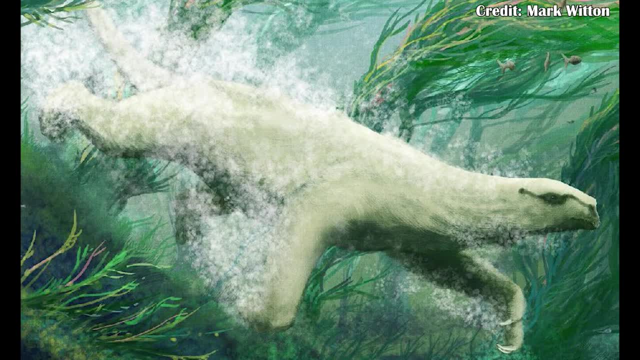 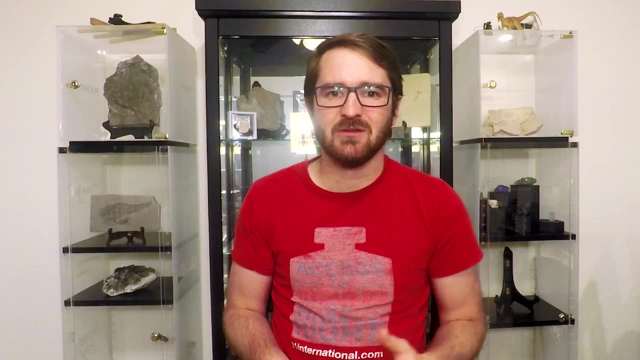 and very adapted to marine environments and grazing on the different kelps that would have been near the shore, And even in modern sloths they're very well adapted to actually swimming relatively long distances, Something that isn't expected of an animal that spends most of its life. 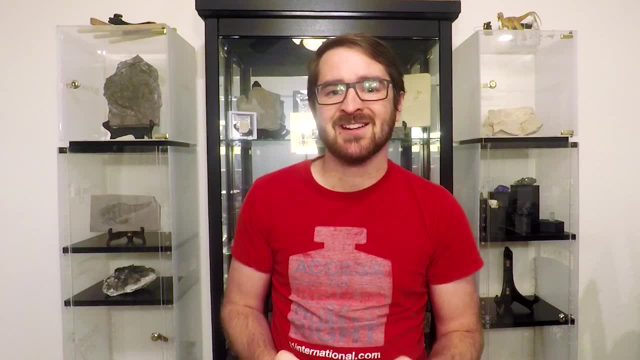 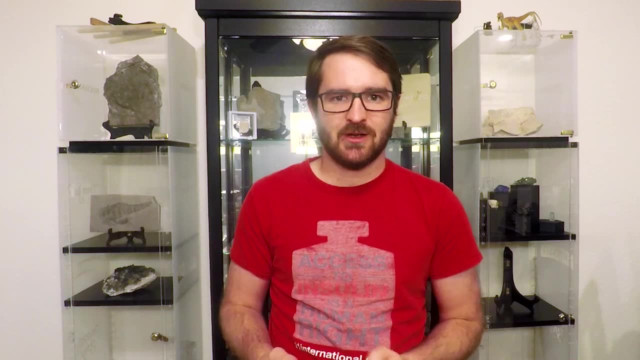 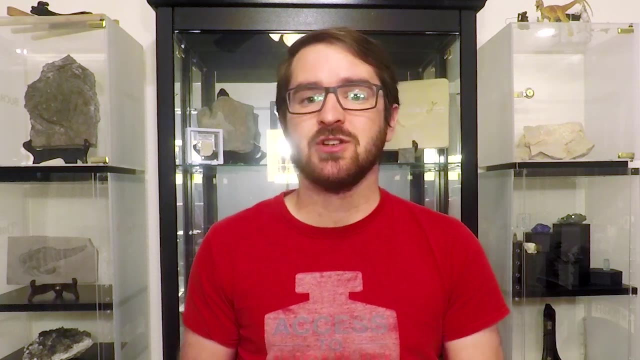 in the water Ground sloths were extinct around the same time a major extinction was occurring in Australia. What a new study on this Australian extinction finds is that parts of it at least, weren't associated with the migration of humans into the continent. Rather, at least in the 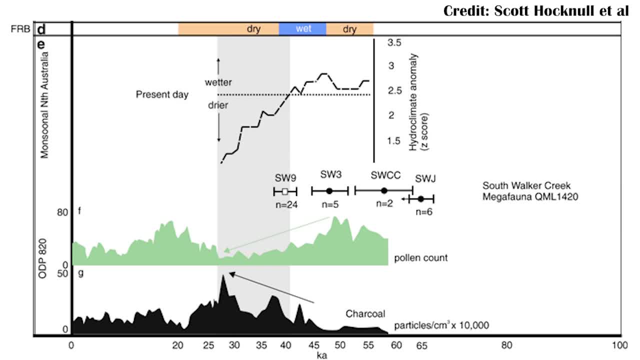 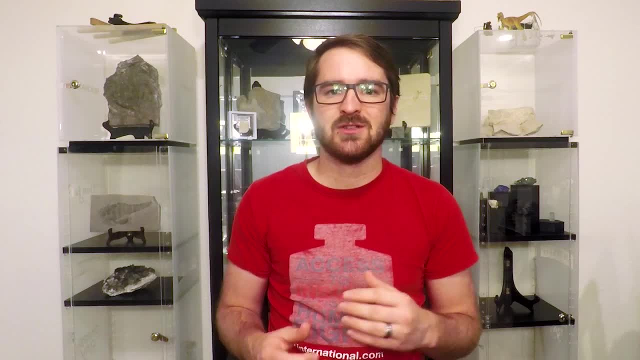 northern part of Australia. it was associated with a long period of prolonged drought. A sequence of rocks coming from northern Australia shows fossils up until a certain point in time, About 40,000 years ago, 8,000 years- into a prolonged drought that lasted up until about. 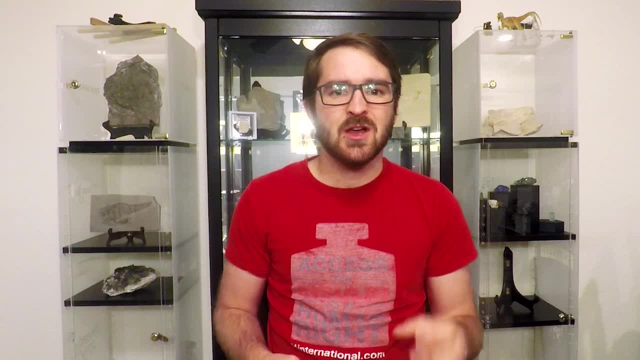 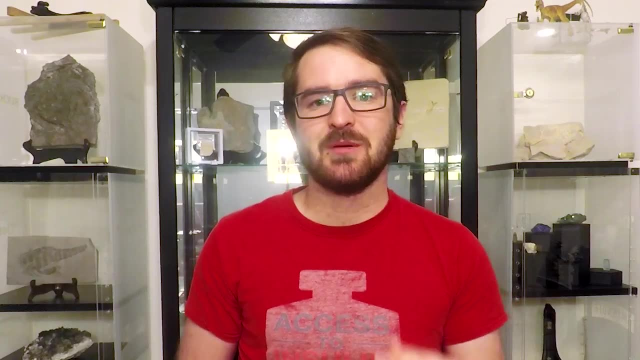 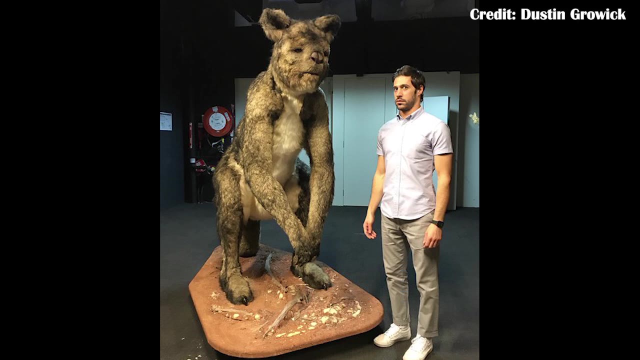 30,000 years ago. Fossils from before this time show even a new species that hasn't yet been described, of the largest kangaroo known. This new kangaroo would have been much more closely related to the modern red kangaroo, the current largest kangaroo, than the animal Procopteron, which is 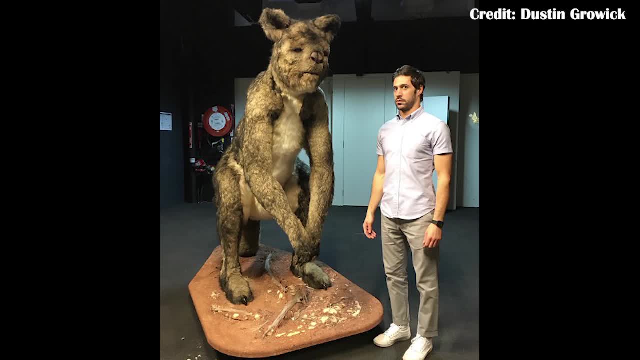 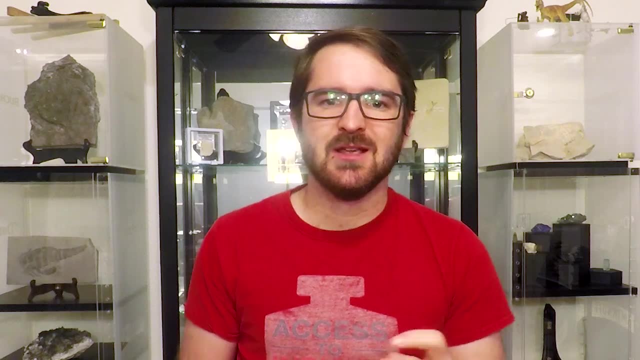 the previously known largest fossil kangaroo and had a much different kind of facial shape. It's a little unsettling. The study does take note, though, that this kind of pattern of extinction isn't followed in South Australia, where it is more aligned with the arrival of humans into the continent. What this 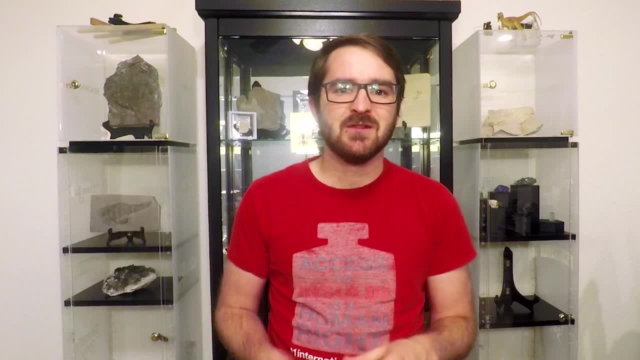 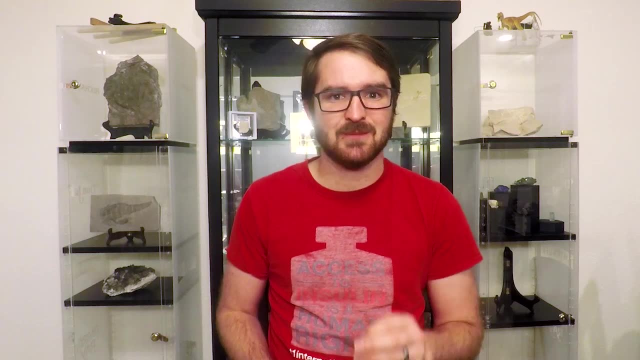 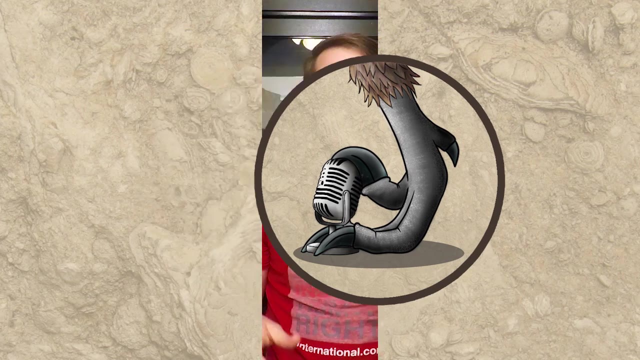 means is South Australia may have acted as a refuge for many of these species from the north, at least up until humans arrived, And that northern Australia did suffer very significantly because simply of the climate change and that very prolonged drought, rather than only from human interaction. Finally, there was one more study on gharials. 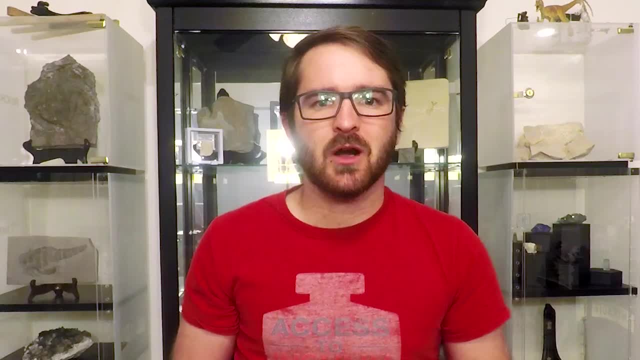 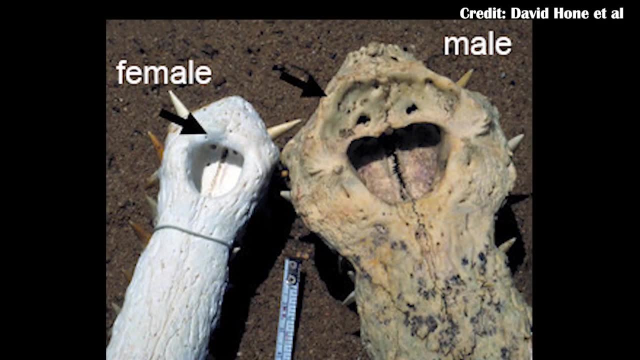 that has very important implications about dinosaurs. Gharials are unique with the archosaurs and crocodilians in that they have a very pronounced sexual dimorphism, with the males having a large bump at the very front of their snout. A new study has sought to see how this 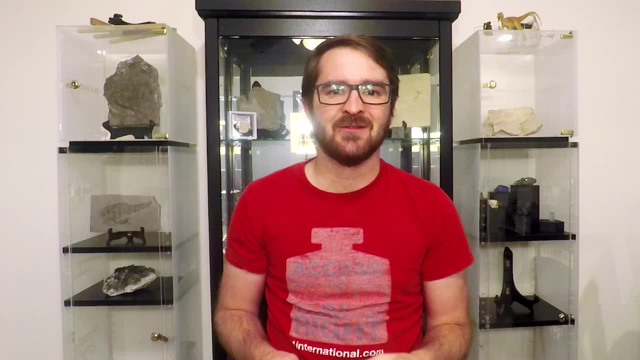 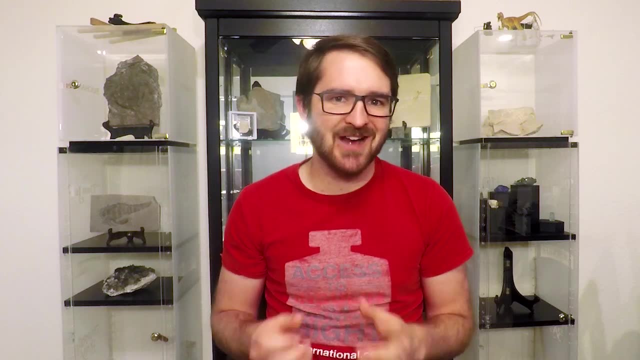 develops in the bone, to see if it would be likely that we'd be able to identify any kind of sexual dimorphism in dinosaurs in the fossil record. What it finds is that it's actually not that likely, at least depending on the age of the animal, While, yes, this kind of dimorphism could be.